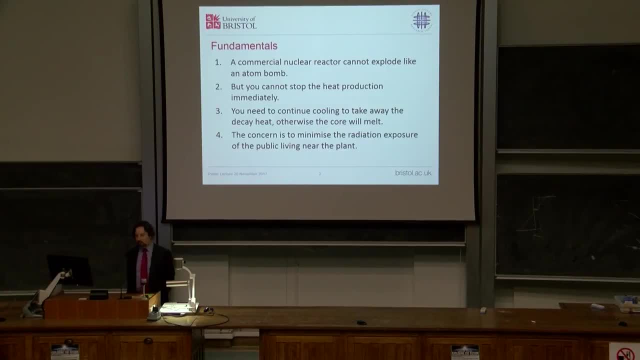 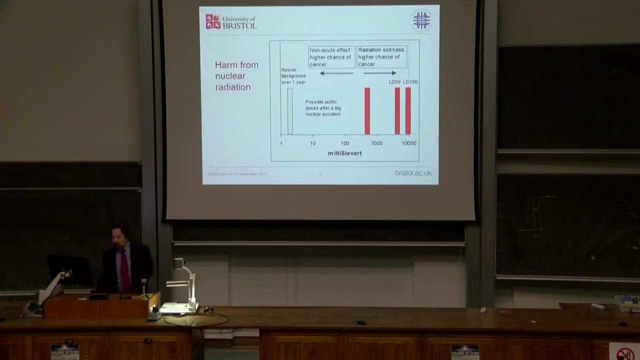 which can then be taken up and deposited around the surrounding area. What you're concerned about is minimizing the radiation exposure of the public who are living near the plant. And again looking now at the harm from nuclear radiation on the right-hand side of that graph in red: 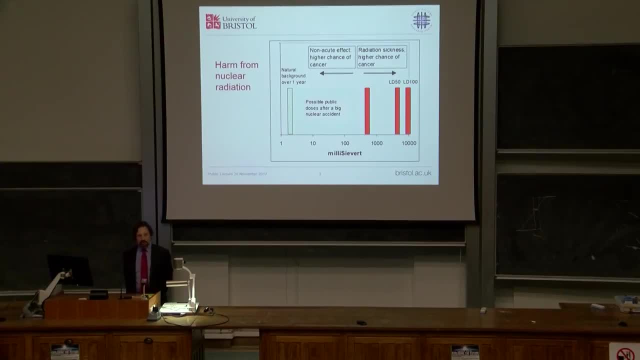 the red bars there. this is where we get radiation cancers- over around about 500 millisieverts. A sievert is an energy term, it's a joule per kilogram and a millisievert is the standard term which is used of that energy deposition. 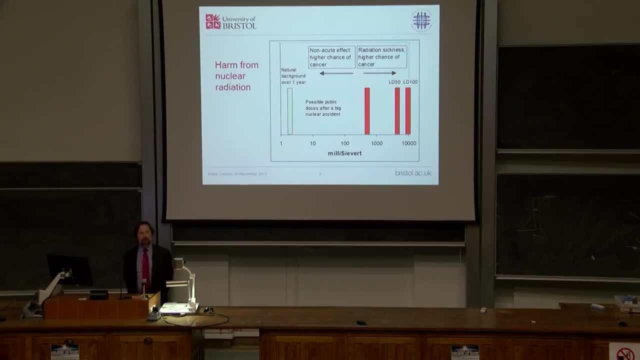 And if that's above about 500, then you can have radiation sickness, That is to say you can vomit, lose your hair and, in extreme cases at the top end, die And the LD there is: lethal dose 50.. 50% of people will die when they get something in the order of 4,500 to 5,000 millisieverts dose in a short time And the lethal dose is somewhere around 5,000 millisieverts And the lethal dose is somewhere around 5,000 millisieverts dose in a short time. And the lethal dose is somewhere around 5,000 millisieverts. dose in a short time And the lethal dose is somewhere around 5,000 millisieverts. dose in a short time And in the range of 100 millisieverts or less, somewhere around 9,000 or 10,000 millisieverts. 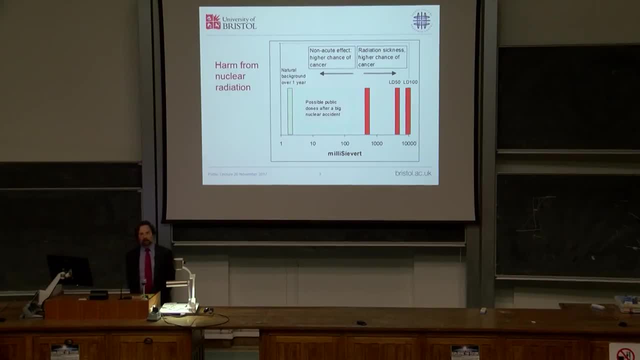 you will be killed and die within a short time hours. but the doses to the public do not lie in that area at all under basically any conditions, And I've put in sort of a slightly fuzzy area there in blue which indicates the possible public doses. 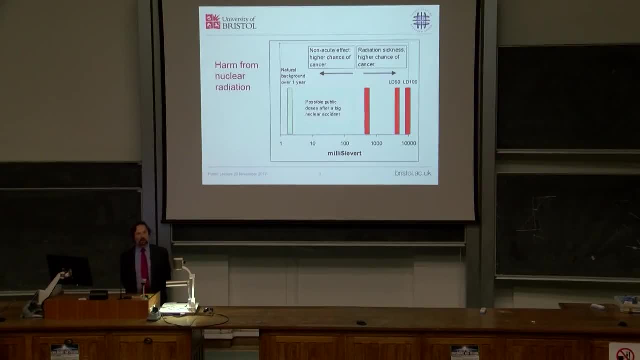 And I've put in sort of a slightly fuzzy area there in blue which indicates the possible public doses. What you're concerned about with these doses is you're concerned about developing fatal cancers, or cancers of any kind, some of which will be fatal. 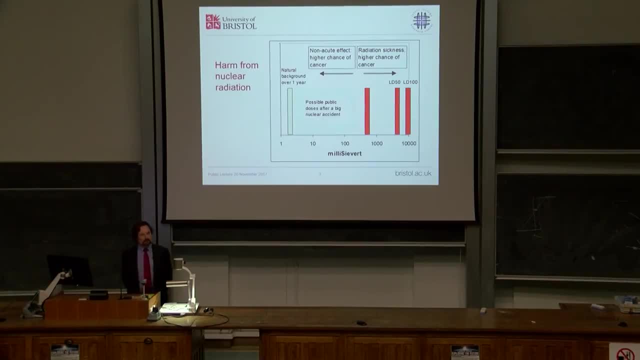 And the probability of developing a fatal cancer goes up as the dose goes up. Meanwhile, down at the bottom in green is the natural background radiation which you'll accumulate over a year, And it's around about 2 millisieverts, and that applies roughly to many places in the world. 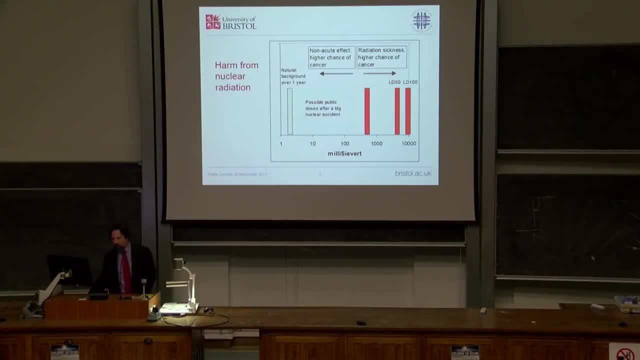 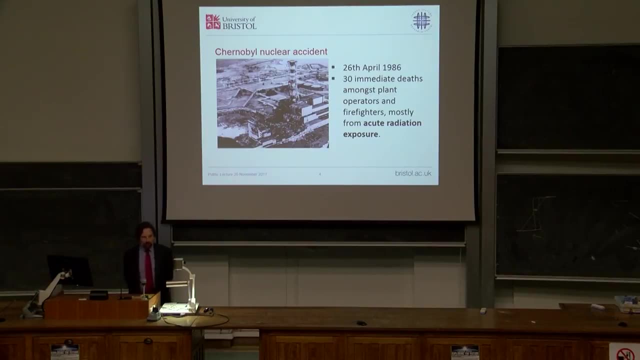 and it applies to the UK Now. the Chernobyl accident is the worst accident we've ever experienced And there the reactor went super prompt, critical, which went the closest it could go to being a bomb. It was not a bomb because 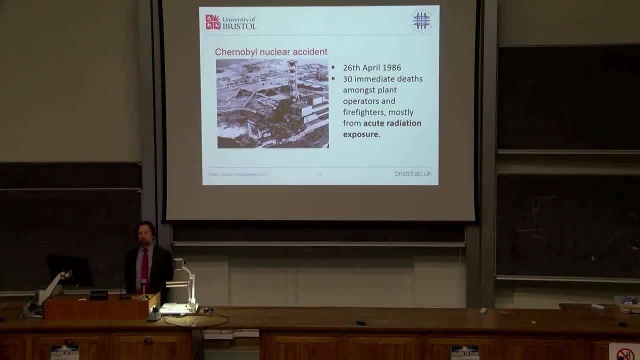 the energy that it released. it didn't release this over the microseconds needed for an explosive. It released this over a period of a few seconds before shutting itself down, And that's the Nordheim-Fuchs phenomenon- that hot uranium is not such a good reactor. and the system shuts down Immediately. But before that, of course, it had melted fuel and that fuel had come out of the reactor. There had been an explosion caused either- probably possibly- a steam explosion and more likely a hydrogen explosion caused by a chemical reaction. And the devastation was very, very significant And, of course, we had a huge, a huge power excursion. 30 people died in the immediate aftermath, 28 more or less immediately and another two from acute radiation poisoning, And they died within three to six months of the event. those poor, unfortunate people there, Mostly from acute radiation exposure. There were some blast effects, There were some burning effects, I believe, But mostly from acute radiation exposure. Now we come to the principal policy response after Chernobyl, which was mass relocation of the public. We want to keep the public safe, Let's move them away from the source of danger, was the thinking, And so a huge number of people were relocated- 116,000- in the days and months after the accident which happened in April 1921,. 1986. And then a further 220,000 were relocated after 1990.. So the total was 335,000. And, as you can see, that corresponds roughly to a city the size of Cardiff. Bristol is a bit bigger. but it would be an awful lot of Bristol would fall into that category and be moved. The Fukushima Daiichi nuclear accident: This happened 25 years later, almost exactly 25 years later, in March 2011.. It was a great earthquake. the Tōhoku earthquake, 80 miles offshore, magnitude 9, huge earthquake. 18,500 people were killed by the tsunami that followed from that, And it caused the reactors to undergo very significant harm. What happened was that they shut down automatically. 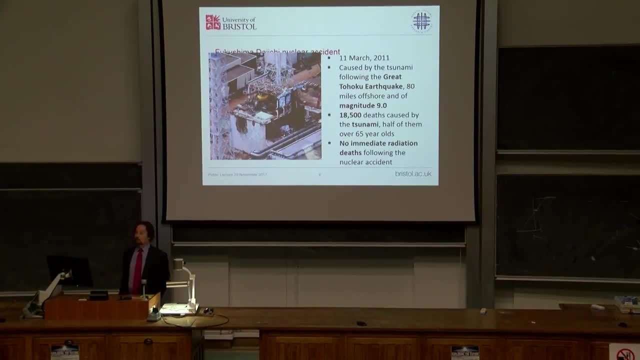 as they should, having detected the earthquake. But that's not good enough because, if you remember the decay heat that I mentioned before, that decay heat needed to be taken away And the problem was the tsunami inundated the pumps that were taking that decay heat away. after about 45 minutes They lost function. So we actually had three reactors melting down And a fourth reactor was actually the fuel pond was damaged And in fact there were four explosions there, A very significant release of radioactivity and hence nuclear fallout. 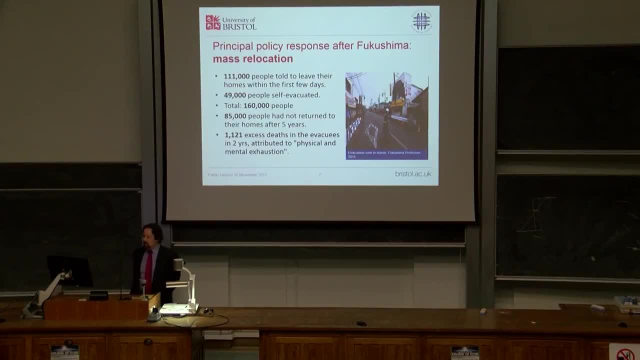 But you'll see a pattern emerging now, And that is that the principal policy response after Fukushima was mass relocation. So Fukushima is a nuclear power plant. So over 110,000 people were asked to leave within a few days And another nearly 50,000 saw what was going on. And they decided to leave anyway of their own accord. The problem with this is 85,000 people had not returned to their homes after five years And probably not many more have returned in the intervening two years since the research that paper. 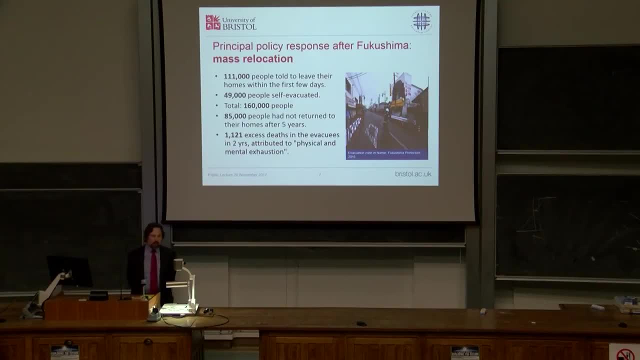 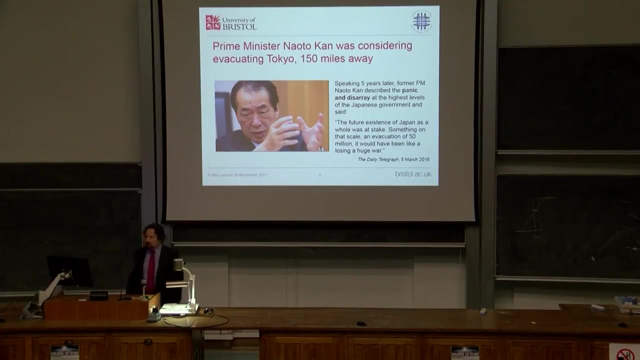 that paper was completed. Moreover, there were a number of people who died of this. These were principally elderly people who died, And they died early as a result of physical and mental exhaustion. Now, the prime minister of Japan at the time was considering evacuating Tokyo. 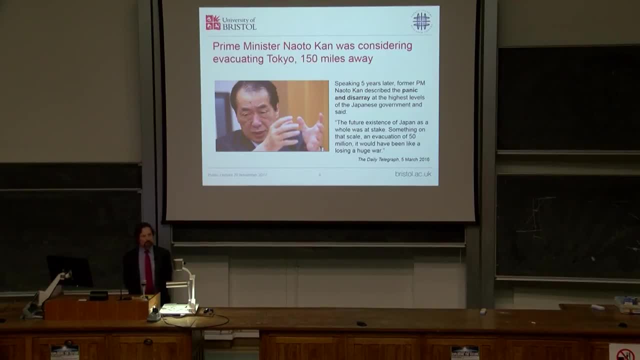 which was 150 miles away. This would have been an enormously enormous decision to take And you can see his comments there. It would have been like losing a huge war. Those comments were made five years afterwards And that was his he's telling of what actually happened at the time. 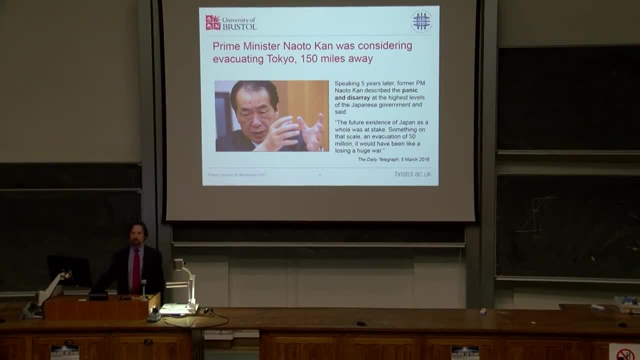 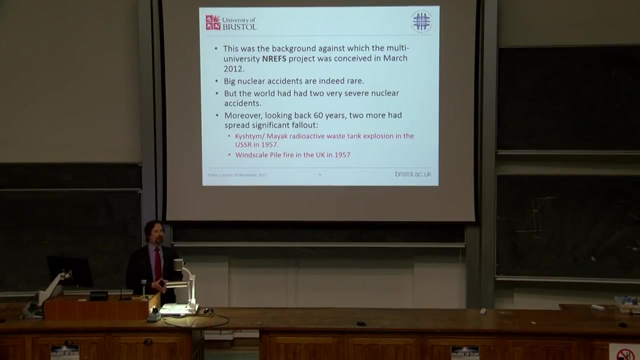 I think the thing to bear in mind there was this panic and disarray which his words quoted in the Daily Telegraph, which the government was in at that stage. So that was the background against which the NRF's project was conceived: Big nuclear accidents. yes, they're very rare things, But we now have had two very, very big nuclear accidents And we've had a few significant accidents to a few accidents that have spread significant amounts of radioactive fallout: The radioactive waste tank explosion, the US SR in 1957.. 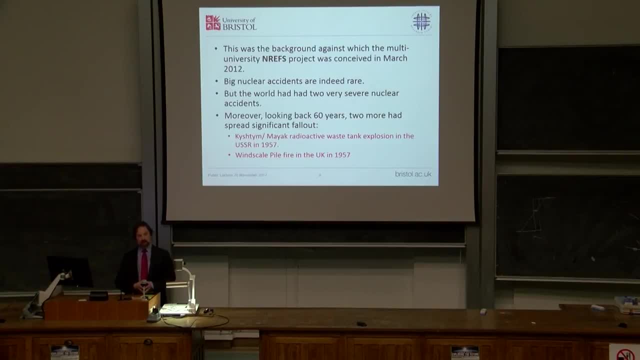 Here in Britain, the Windscale Pile Fire in the UK where a reactor, one of the first generation, very simple reactor which was there to produce plutonium for nuclear weapons- That underwent a fire because the Vigna energy had not been released. 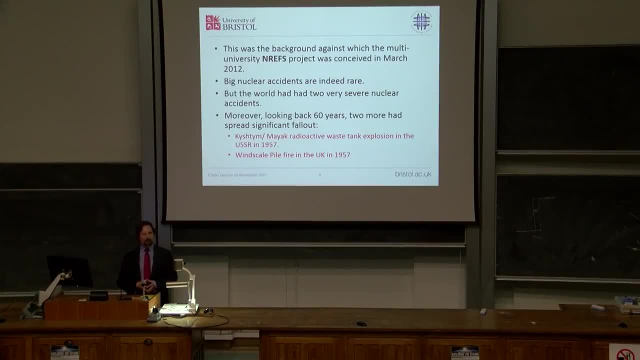 Essentially, the metallic fuel had not been annealed And it came out in a rush And then a fire occurred. There was a widespread release of radioactive material into the atmosphere. So the question that we were looking at was: how should we cope after a big nuclear accident? has actually happened. One of the worst- as bad as it gets as far as nuclear is concerned- Is mass relocation and abandoning of homes. is that the best strategy It's been used in now two big nuclear accidents that have happened in the world? 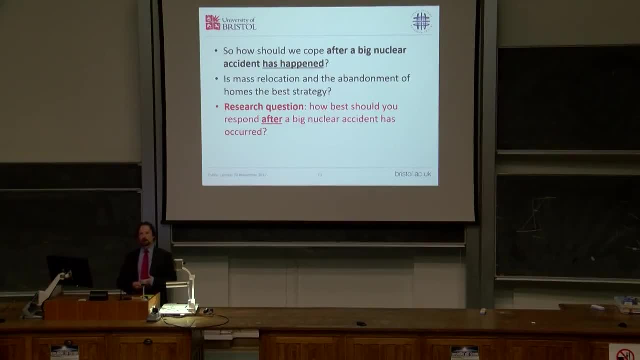 And then, more generally, the research question was: how should we respond after a big nuclear accident has actually occurred? The NRES project, which the Dean has described, there four universities and continued here at Bristol. I think it may not perhaps be a surprise. 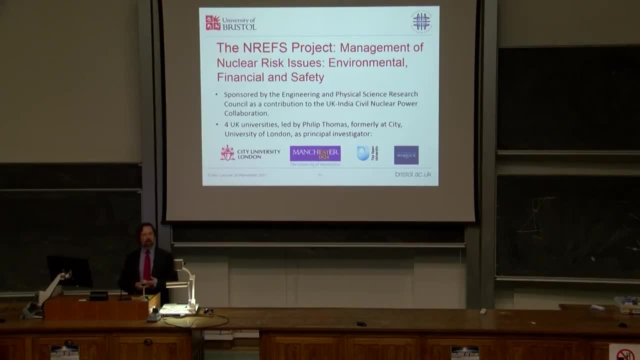 that once one has actually finished doing the actual research. translating that into the final set of research papers is never a trivial, nor often a very short task. But that has now been completed and we have publication of that, Of those papers, of ten papers. 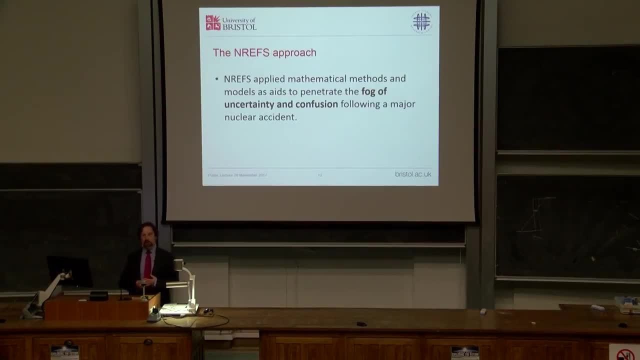 which are there in Process Safety, Environmental Protection, a special issue of that journal. The feature of the NRES project was it decided to attempt to apply mathematical tools and it was clear from what had gone before that what was needed was something to help alleviate the fog and confusion. 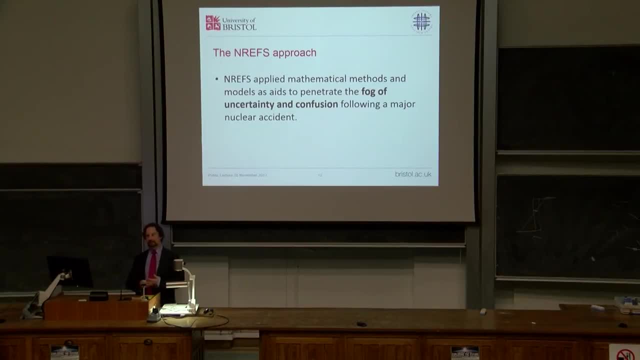 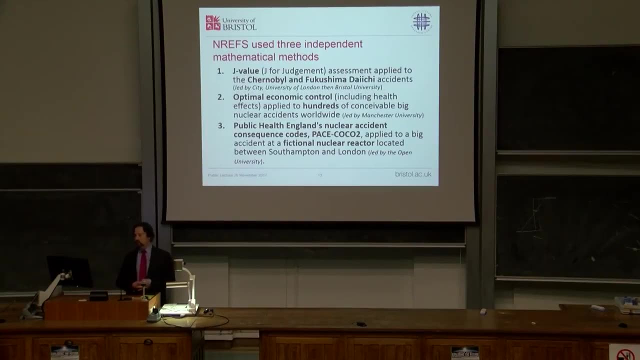 that naturally occurs after a big nuclear accident. Another feature was that we actually used in the NRES study. we used three independent mathematical methods- The J value, J for judgment- and I will say a bit more about that in a moment. I will describe each one. 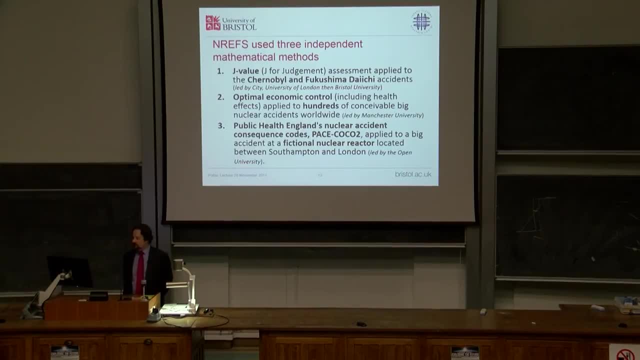 to a certain extent, The J value assessment and we applied that to Chernobyl, these two big nuclear accidents, to Chernobyl and Fukushima, on a retrospective basis, that if we knew now what we knew, sorry, if we knew then what we knew now. 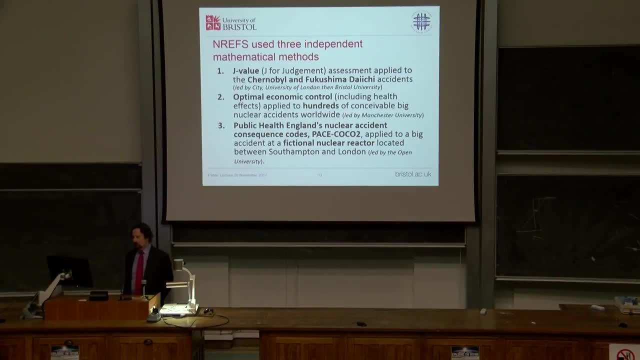 what would we do? Would we still do those things that were actually done? And then optimal economic control, which actually included health effects, were applied to hundreds of conceivable nuclear accidents all over the world. That was work that was led by Manchester University, and then we applied the codes. 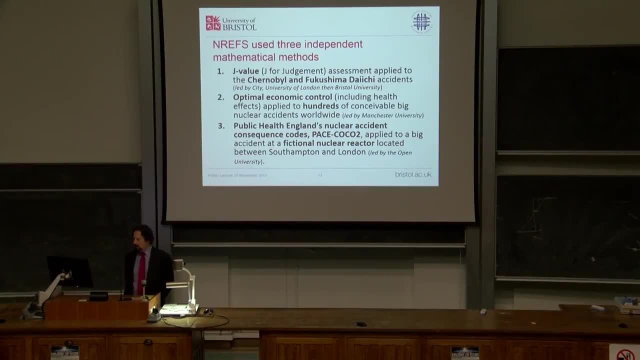 that had been developed by Public Health England for looking at consequences of nuclear accidents and the costs associated with those consequences, And we applied that to a big nuclear accident assumed to occur on a UK reactor located in a fictional site halfway between Southampton and London, and that was led. 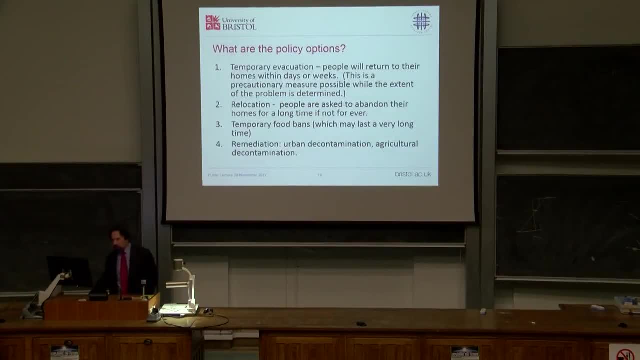 by the Open University. So what are the policy options? First of all, we need to get people back on their homes, and we need to get people back on their homes within the next three months of a nuclear evacuation, but this is really something which is quite short term. where you might move people out on a precautionary basis, but you would get them back within days, or at least certainly a week or two. Then, moving on relocation, which is what's happened before, and people have been asked to abandon their homes, either forever. or at least for a very long time, with all the consequences that that brings about. If you can imagine you've been away from home for five years, how much do you really want to move back to that? So relocation, food bans- temporary or long lasting? 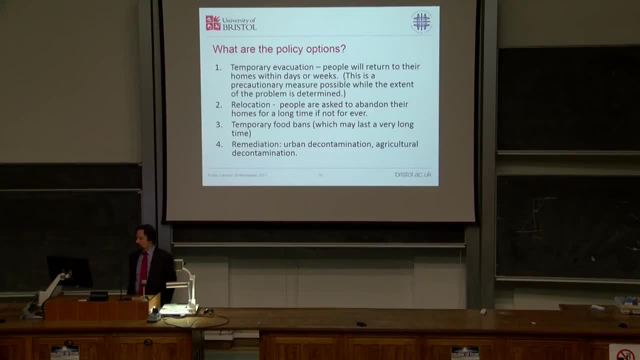 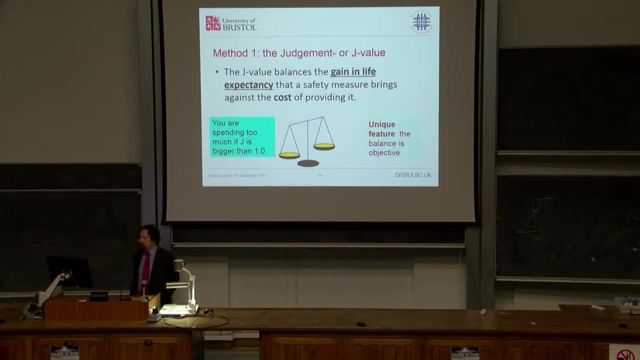 or even in the limit, permanent and then remediation. So this is cleaning up urban decontamination, agricultural decontamination. To talk about the first method, the judgment or J value. what we're looking to do there is balance, the life expectancy. 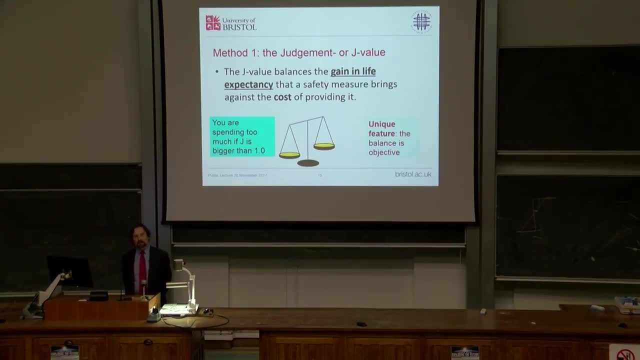 that a safety measure brings with it against the cost of providing that safety measure. And it's that balance that enables us to say that if the J value- we take J as being the ratio of what you are spending or what you're considering spending, compared divided by 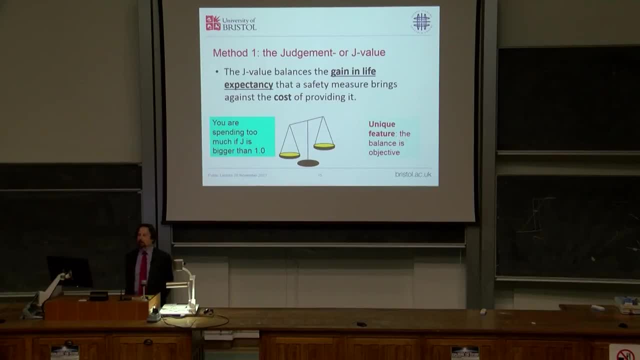 what you, the maximum that you ought to be spending, And that tells you that if J is greater than one, you're spending too much. And the unique feature of this is that it is entirely objective. There is no opinion involved in it. 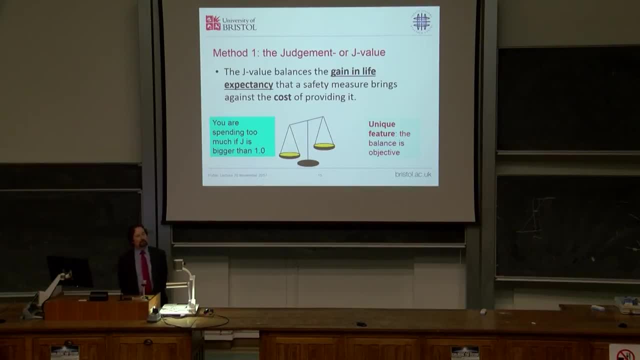 It's based on data from millions of people, both actuarial data, life statistics, life tables, and also on millions of people and economics. So it's economic and actuarial data and it is completely objective. That is to say that any team around the world 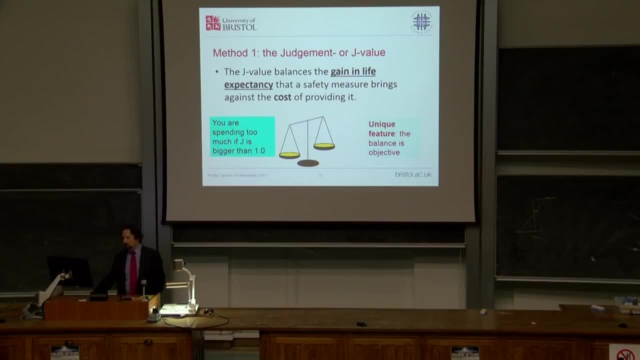 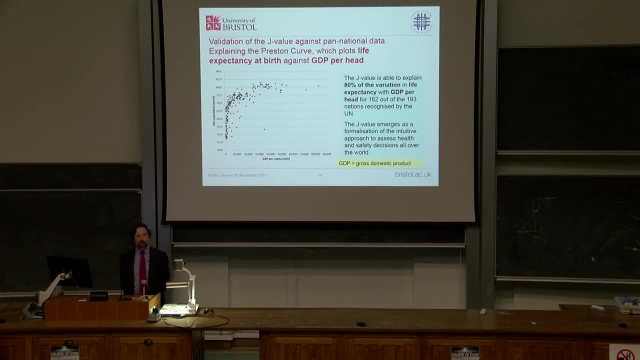 could use that same method and they would come up with the same answers. One of the things that we did during the development of this was to actually validate the J value against pan-national data, And what we were able to do was to explain the Preston curve. 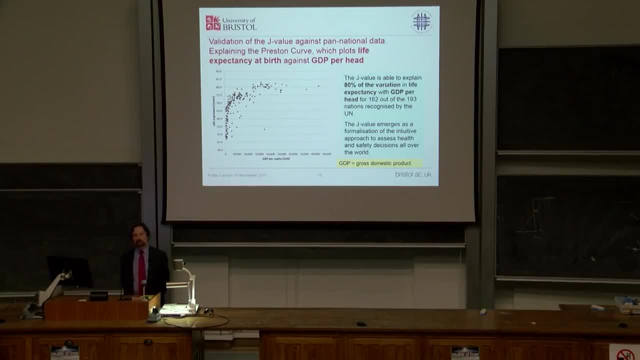 The Preston curve. Samuel Preston in 1975 pointed out that GDP per head has a huge influence on how long people live at birth. And that's the graph for 180 countries in the UN, 193 in the UN, And that graphs the life expectancy at birth. 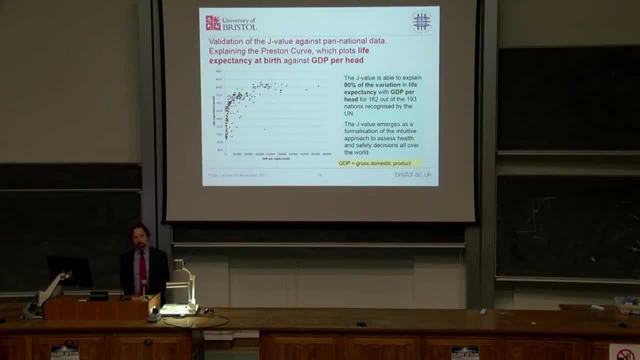 And we were able to explain that, and we were able to explain 80% of the variation between countries, which is a pretty high figure for any social science study, which this effectively is. in this instance, We did that for 162 out of 193 and 60% if we actually looked. 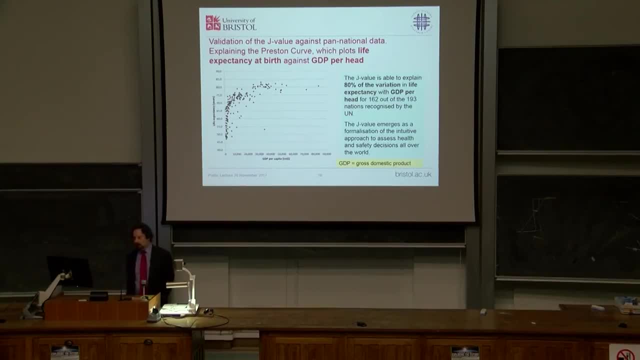 at the full set, on which we had data 180.. And what we found was that the J value emerges as a formalization. It's what people do. basically, it describes how people take their decisions on safety in all countries, in all areas of the world. 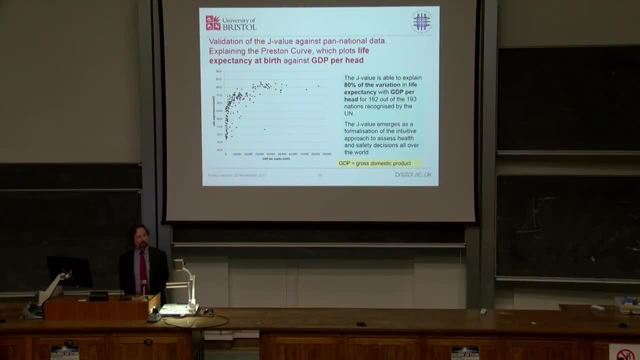 taking into account the resources they have available. That is to say that if we were in any other country in the world, we would act pretty much as those people act And we would take the decisions that those people take. I'm going to mention 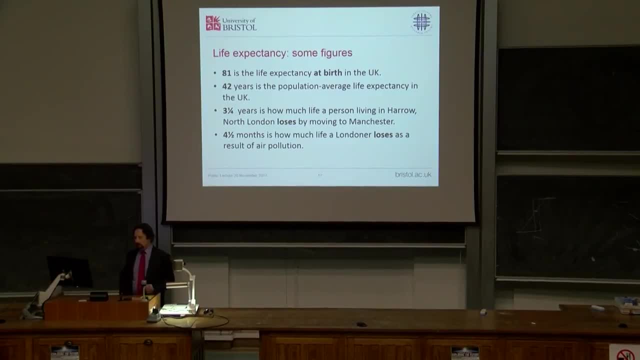 some figures on life expectancy, because I'm going to talk quite a lot about life expectancy, so it's a good idea to put something concrete down. The life expectancy at birth in the UK is around about 81 years. Excuse me, 42 years is the population average. 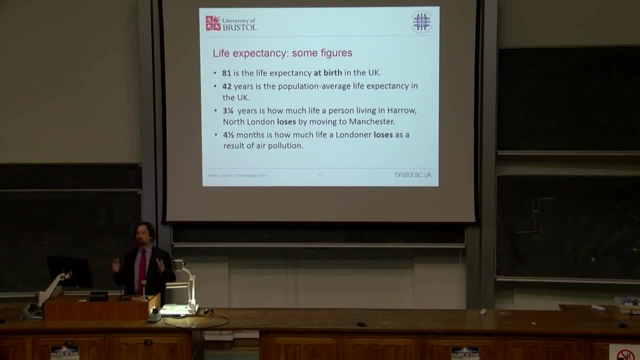 So if we actually take everyone's, how long is everyone going to last from now? if we looked at the whole nation, we'd say, well, people are going to live, on average, 42 years before they die. It's average across all ages. 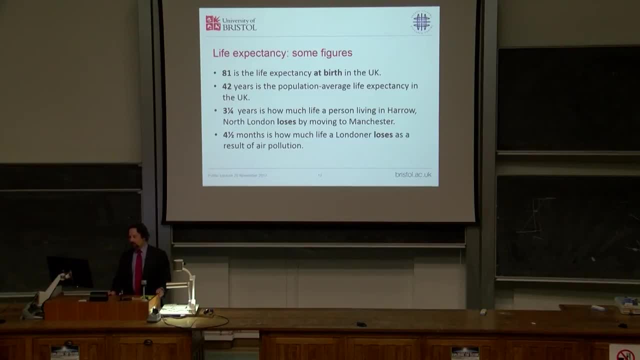 Now let's come down to some particulars here, And this one was something which always upset my colleagues at Manchester. It just happened to be so. I happened to be working in London, They were working in Manchester, Three and a quarter years lost by someone who moves from North London. 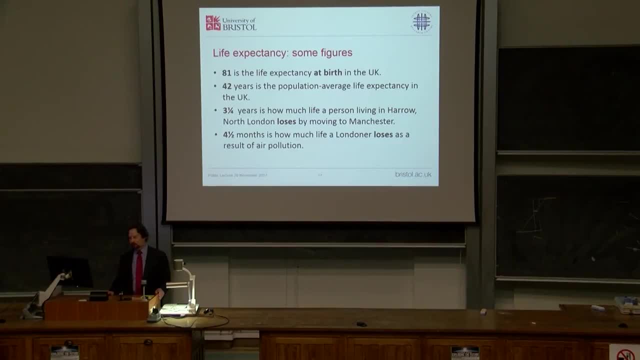 in Harrow in North London to Manchester. That's the average person, And it's six and a half years if you do it at birth, And then four and a half months is what the Londoner, by contrast, loses to London's air pollution. And that's on average across the population. It's nine months at birth. Now let's look at some. to put things in context, let's look at some losses of life expectancy after the Chernobyl reactor accident. Well, we in this country, looking at the standard way of calculating the harm caused by radiation, we lost just under three hours of life expectancy in this country because we had some fallout in this country. Well, the 116,000 people who moved away, how much life expectancy did they lose? Less than 10 days. But that's not the question. The question is what would have happened to them if they had actually stayed in position, Those 116,000 making up the first relocation? Well, 85,000 of those people. would have lost on average just three months life expectancy. So if the world's worst nuclear reactor, 85,000 of the people in that first evacuation would have only lost three months life expectancy. that's only two-thirds of the figure that people in London are losing as I speak. 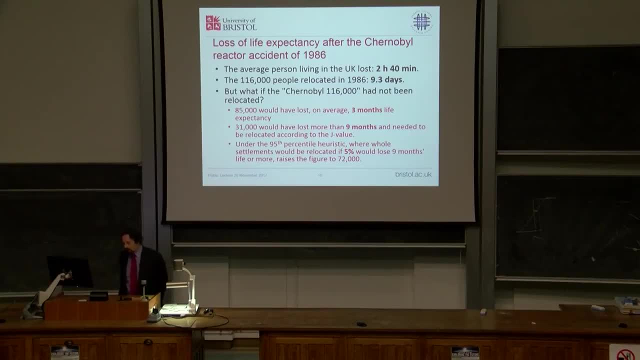 31,000, would have lost more than nine months life expectancy And according to our method, the J value- we would say they ought to move out. It is worth it for them. And if we actually stipulated that whole villages or towns, settlements, needed to be relocated. if 5% of those people needed to be relocated, that is to say their loss of life expectancy was nine months or more, then the figure would rise to 72,000.. But that's still quite a lot less than 116,000. Now let's move on to the second mass relocation after Chernobyl. Now, 220,000 people were relocated. This is four years later. Why did they do this? Well, 220,000 people were relocated after 1990.. If we look at the most highly exposed, 1,000 of those. 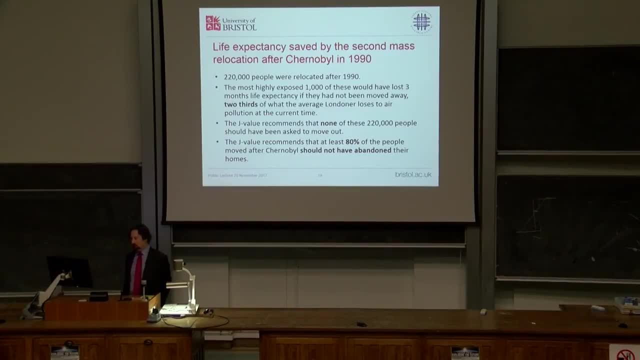 they would have lost less than three months life expectancy. So, not surprisingly, the J value recommends that you shouldn't have moved any of those people. So, in total, 80% of the people who moved after Chernobyl accident should not have been. according to the J value, 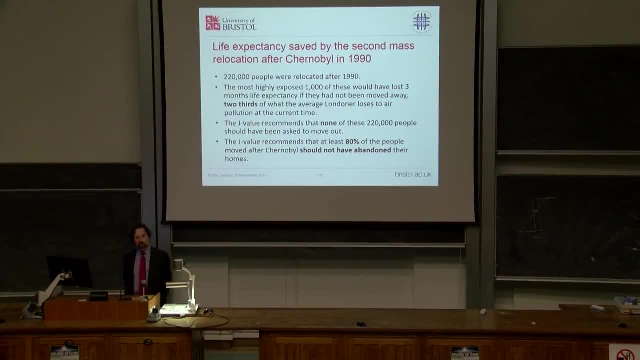 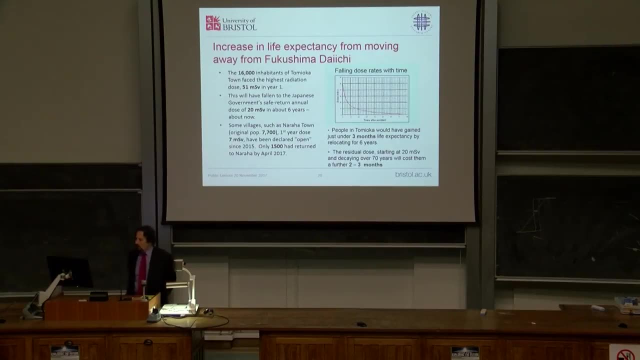 That's, a city the size of Derby should not have been moved. Now let's have a look at Fukushima Daiichi. Well, Fukushima Daiichi was by no means as serious an accident as the calamitous accident that happened at Chernobyl. The worst affected people there 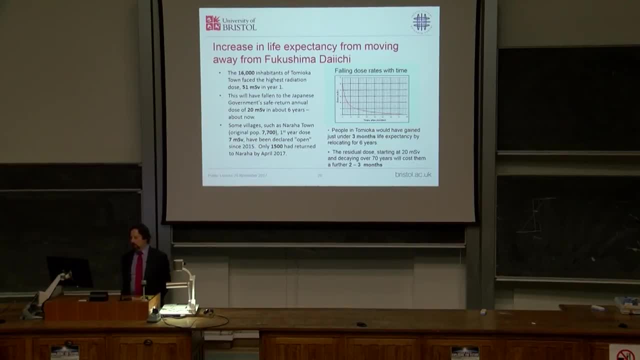 were inhabitants of a small town called Tomioka And they faced the highest radiation dose in year one, But it was only 51 millisieverts over the whole of that year And that will have fallen to the safe return dose, which is what the Japanese government has stipulated. 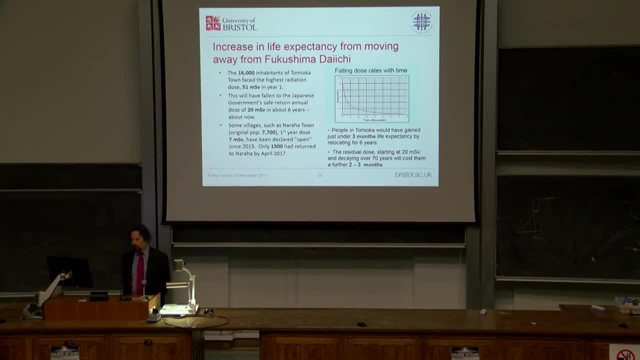 20 millisieverts per year After about six years- that's about now- Some of the villages started off with less dose than the 20 millisieverts per year safe dose. One of those is Naha Raha town, But you see there that people moved out. 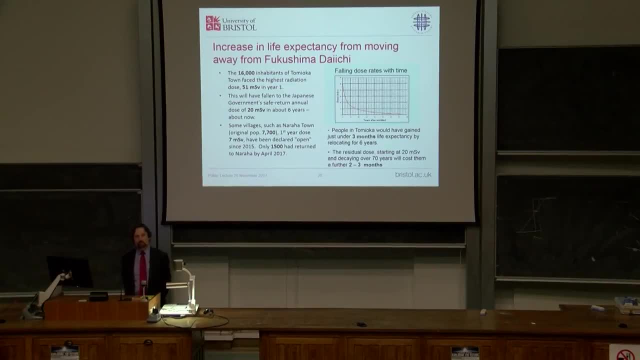 And very few have moved back. So what was the benefit of moving out For people in Tomioka who were the most exposed, then they would have gained somewhat less than three months life expectancy by relocating for six years. And if they then over and having come back, 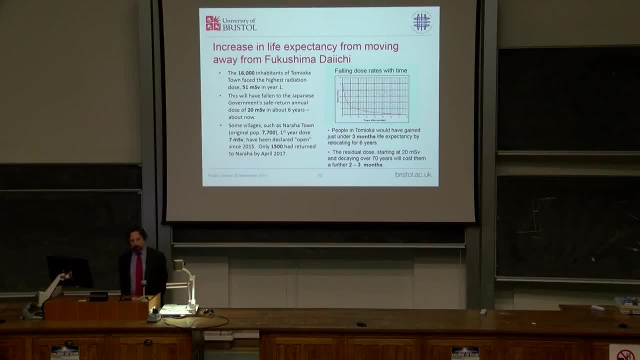 they would then lose a further two or three months from the relocation, Living under the safe relocation dose. One of the things about this is that the dose is falling away at all times, And that's what the graph on the inset graph on that shows you. 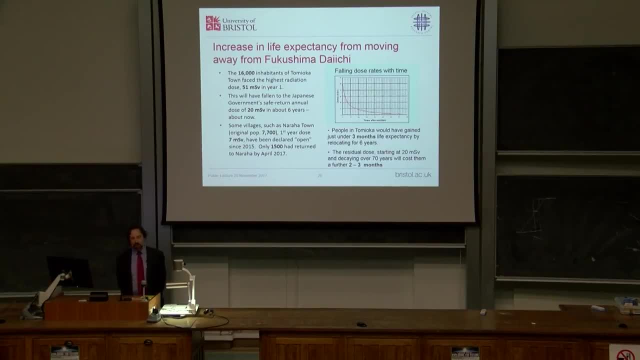 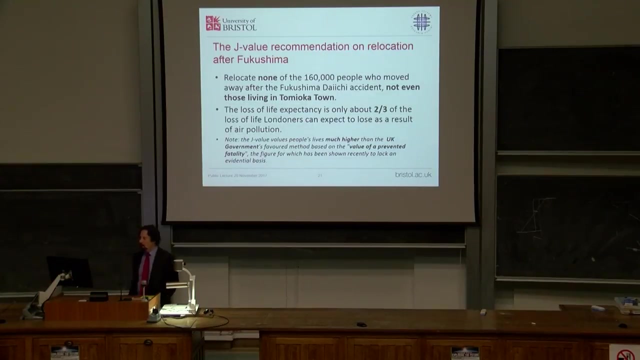 But if you get, it's 51 millisieverts in year one, but it's falling away very rapidly and is a lot, lot lower by year five and year 10 and so on. So was it worth it? No, As far as the J value is concerned. it's difficult to justify relocating any of those 160,000 people who are relocated after Fukushima, the accident at Fukushima Daiichi. That's what the J value recommends And, to put it in context for intuitive purposes, we're talking about less than two thirds. 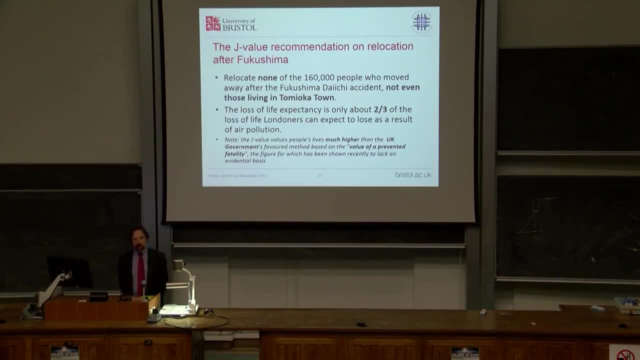 of the air pollution toll on Londoners And if you think the J value is accurate, it's actually encouraging people to take risks. I can tell you that it's a lot. it values life much higher, much, much higher than the UK government's value. 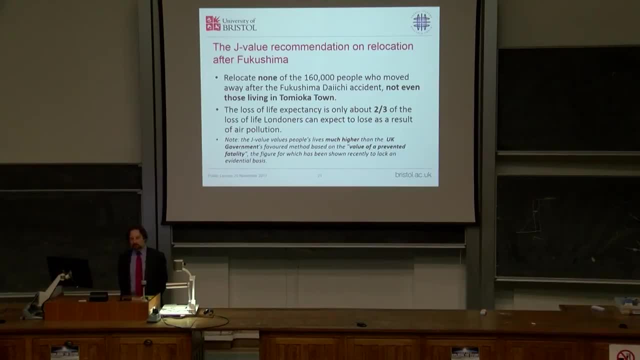 of a prevented fatality, which is the standard method for cost benefit analyses in the UK. That has its own problems, which have been pointed out, And it is but in addition to that, even if we put those problems to one side. 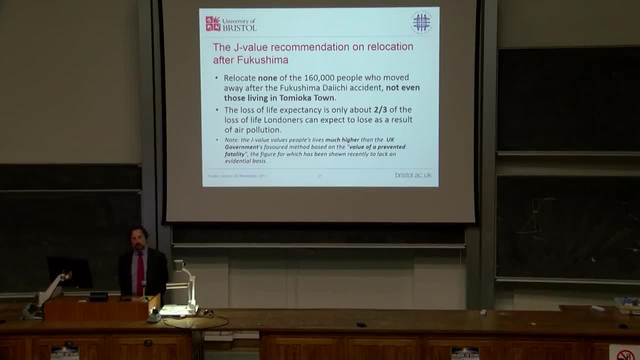 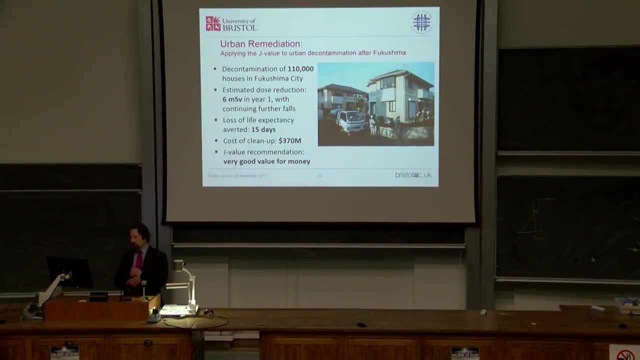 the J value values life a lot higher, So these are not soft recommendations. When it comes to urban remediation, then the things that are being done are quite sensible. So the decontamination of 110,000 houses in Fukushima City, that was a good idea. It cost $370 million but it's good value for money. The agricultural remediation: here again, at least even 20 years after the accident. then agricultural remediation like aniline ferricin to cattle feed to reduce the uptake of radioactive cesium. 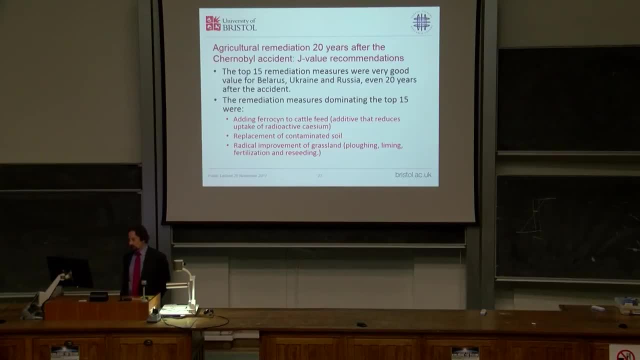 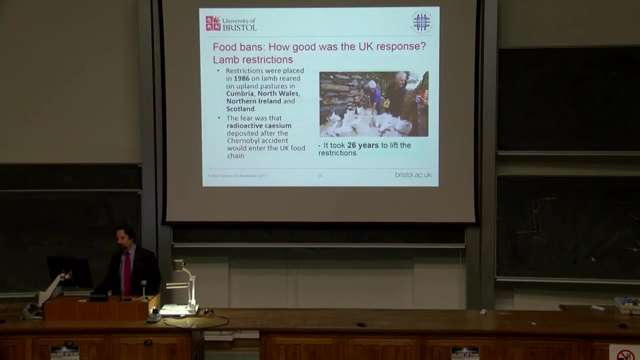 which is the principal component. that is the problem: Replacement of contaminated soil and then ploughing liming and so on. Again looking to substitute, to displace radioactive elements with similar elements, chemically similar and stable elements. But they're a good idea. 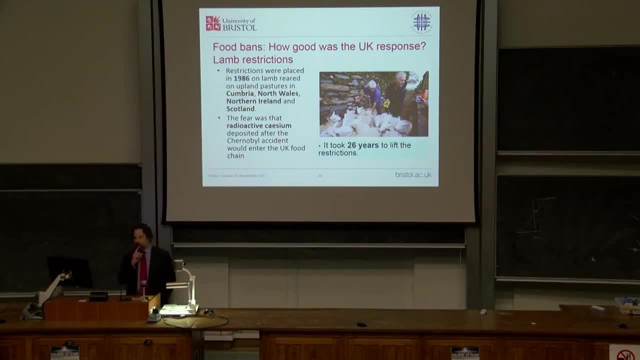 Food bans- We ourselves. how did we fare after Chernobyl? How did we do? We actually looked at these. Obviously, there were a number of things we could look at. There was a huge number of things we could look at. 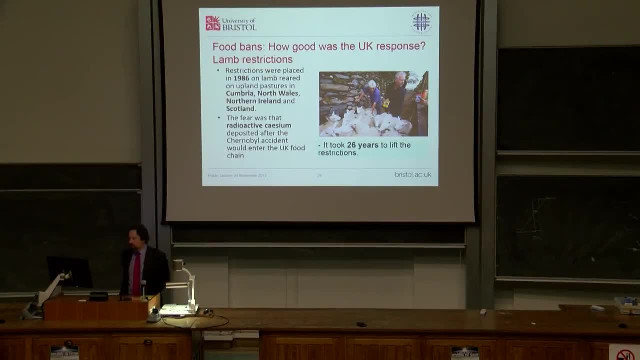 but we were restricted in the amount of time we had, But we did look at the UK response on lamb restrictions. The problem with that was that it took 26 years to lift the restrictions And so banning lamb from certain pastures from entering the food chain. 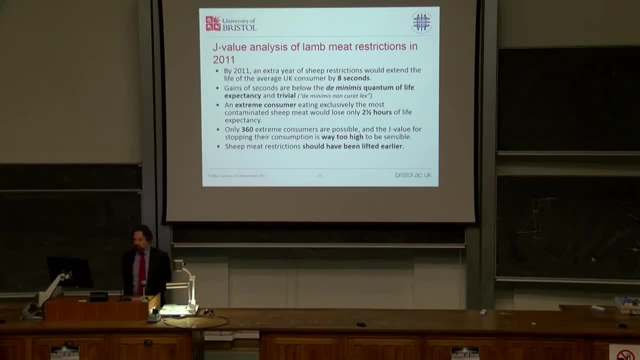 it took 26 years before they were removed And by that stage they were saving eight seconds of life for the UK citizen, which is not very high, I think you will agree. An extreme consumer who eats loads of contaminated sheep meat only contaminates sheep meat, basically. and he'd lose two and a half hours of life expectancy. So the sheep meat restrictions should have been lifted earlier. I want to throw this one in to give some indication, because I've talked about loss of life expectancy and I've talked about it across a population. 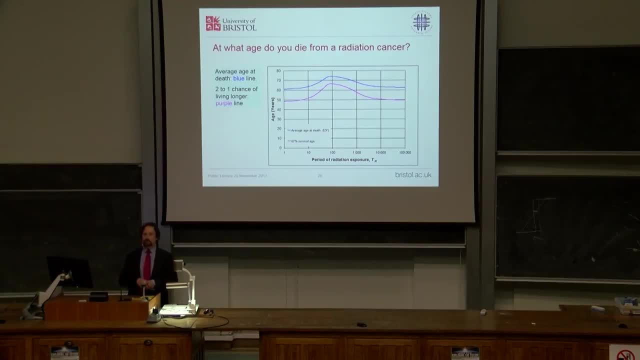 which is an average across a population. But what happens to those people who, those poor people who actually die as a result of the radiation that they get? They die as a result of a radiation cancer. What age do they die at? Well, the blue line shows their average age at death. 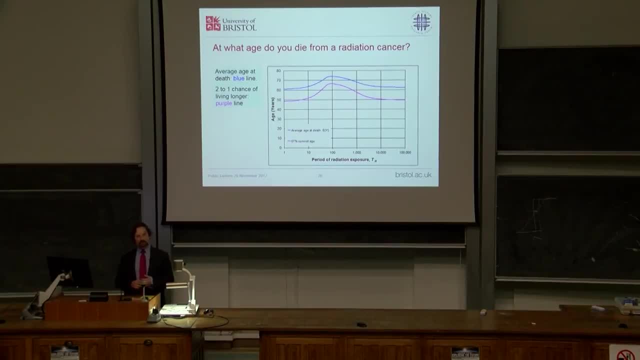 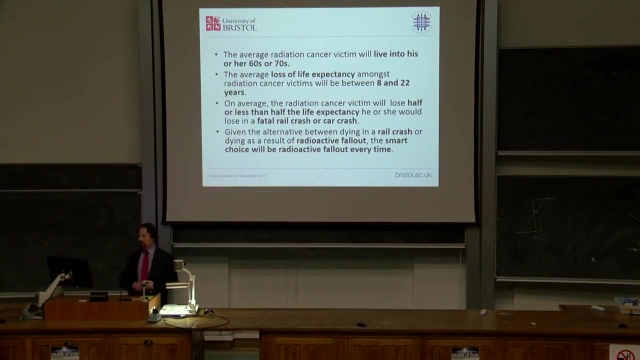 And you can see from that that they will tend to live into their 60s and they have a two to one chance of living longer than about 50. So that's a further thing for you to think about. And then the loss of life expectancy. 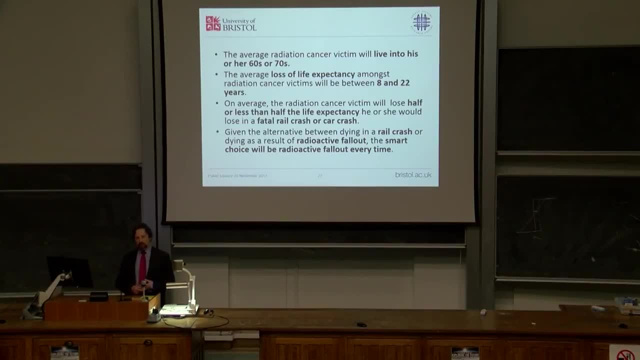 for a radiation cancer victim is between 8 and 22 years. What that means is that, on average, the radiation cancer victim will lose half or less or half or less than half the life expectancy he or she would lose in a fatal accident. 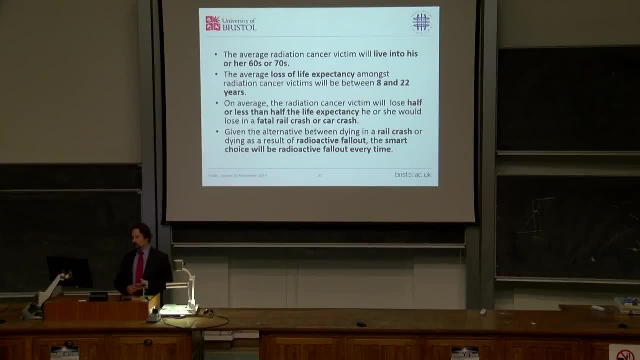 such as a rail crash or a car crash. So there's a certain amount of gallows humor. perhaps you might think in the last sentence there: but if you did have a choice, it's an unrealistic choice, but if you did have a choice. 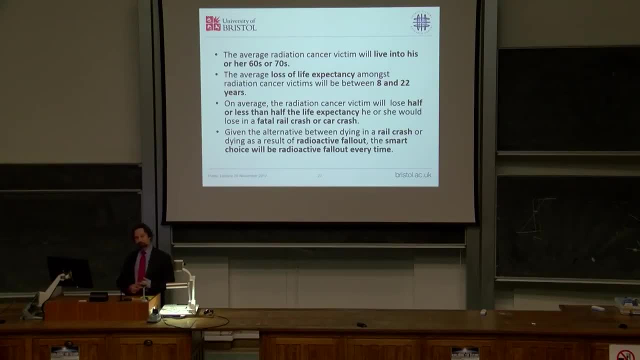 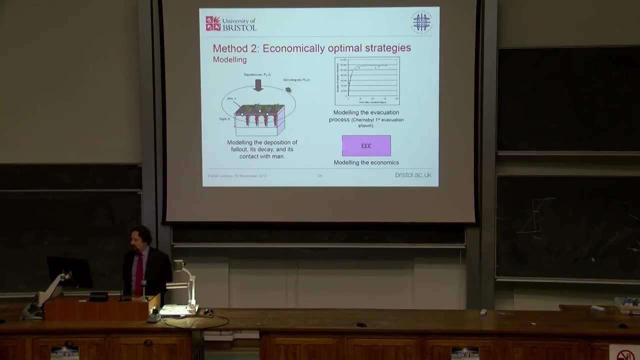 then radioactive fallout every time. Second method we looked at was to develop economically optimal strategies modeling the deposition of fallout, its decay and its contact with man in a fairly simple way to get a tractable model that could be used as far as optimal economic control is concerned. 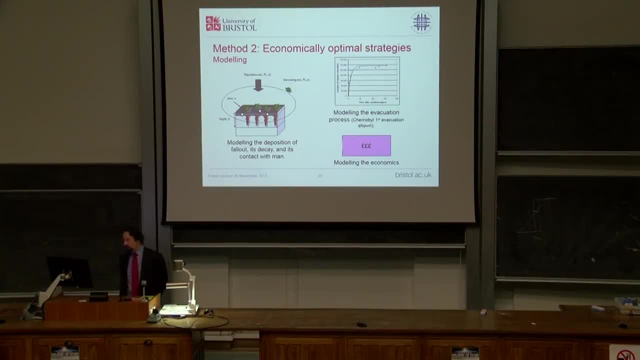 modeling the evacuation process, that's the Chernobyl evacuation process and the dots on that graph, and then the line is the actual model and then modeling the economics. Four hundreds of potential accidents at nuclear reactors spread all over the world, And the method that was used was 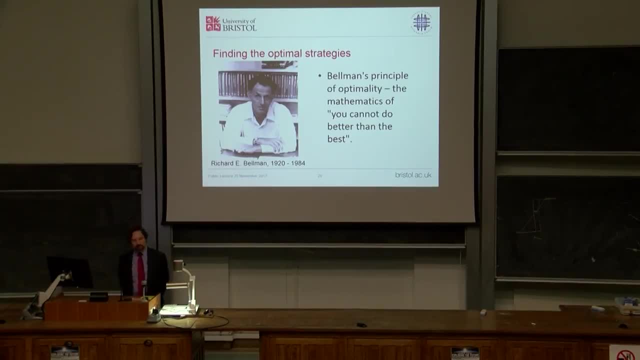 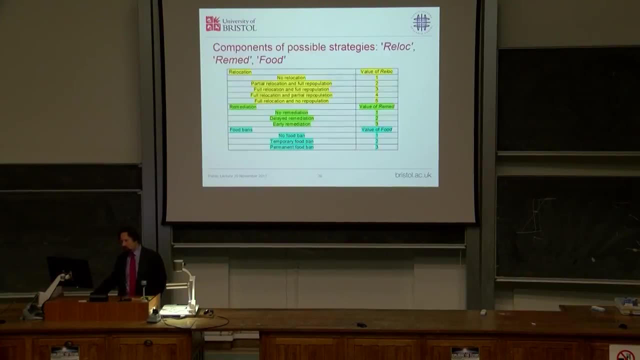 Richard Bellman's principle of optimality, which is basically the mathematics of: you cannot do better than the best. Very often, mathematics is concerned not so much with discovering new things, but is it proving that what you knew all along was sensible and, in a sense, 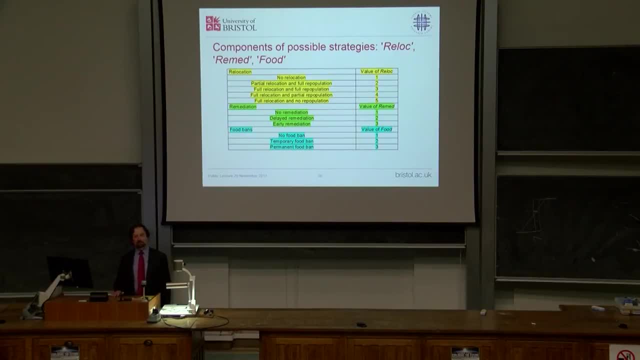 that's when Bellman talks. Bellman's principle is in a sense like that, but the mathematics to derive it, then spread it and apply it more to many problems can be rather complex, which is why we had Manchester mathematicians to do that for us. 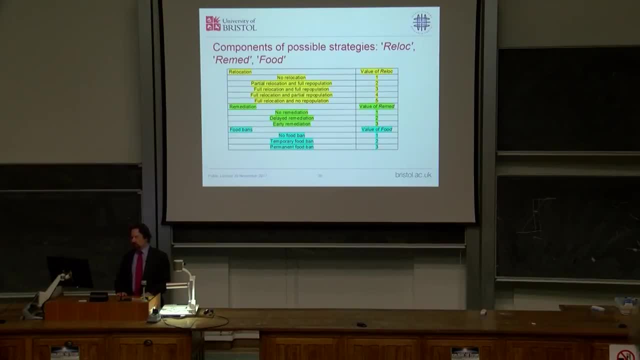 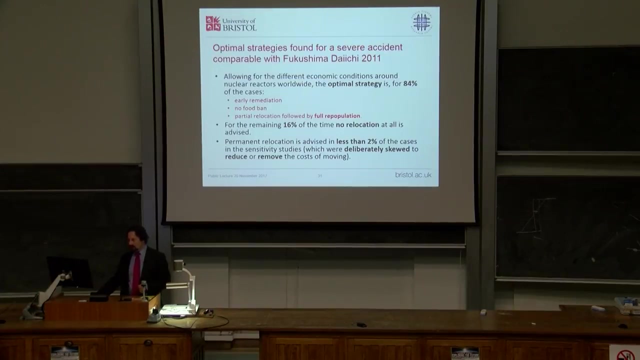 And a number of strategies were put together and those illustrate the five possibilities under relocation, three possibilities under remediation and then three possibilities under food bans. And so that's the spread, and that was the way in which these things were looked at For most cases. 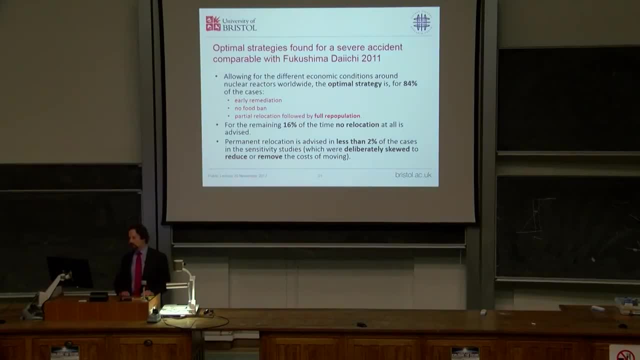 for these hundreds of cases that were looked at, the optimal strategy was to carry out remediation early, not to ban foods and to relocate on a partial basis, but then follow that up by full repopulation And then for the remaining time. don't relocate at all And permanent relocation, such as we've seen at Chernobyl and such, is de facto what's happening at Fukushima. that's only a good idea when you skew the cases to reduce or remove the cost of moving. 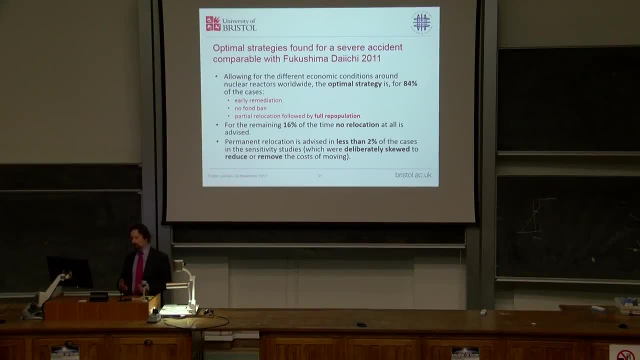 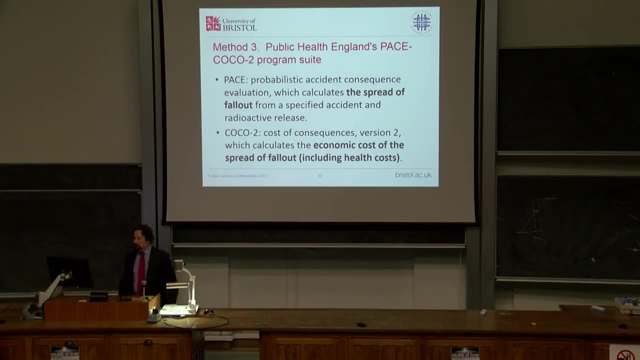 which is a somewhat more unlikely case, and even in that case it's only 2% of the cases. And then method three was the Open University, which used Public Health England's PACE-COCO2 program suite and looking at the spread of fallout. 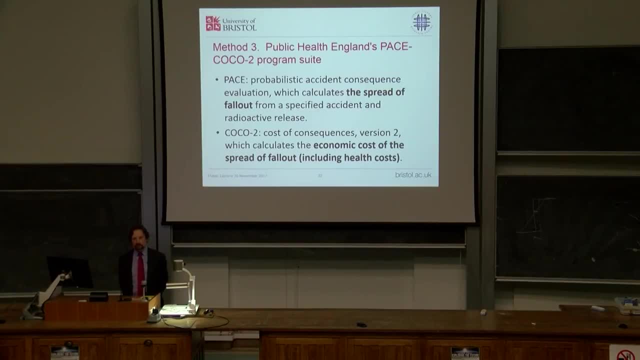 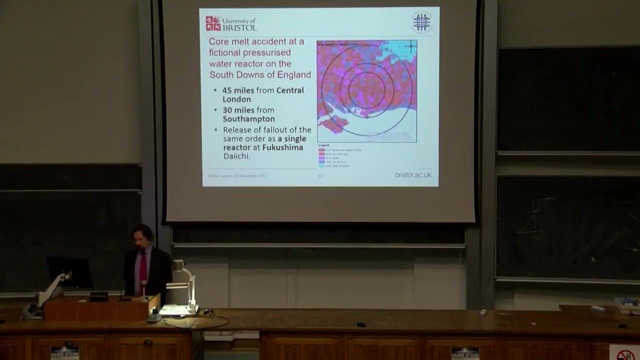 from this reactor 45 miles from central London and 30 miles from central Southampton, And finding out the economic cost- and that includes the health costs- for that. The idea was that a core melt accident occurred at a fictional pressurised water reactor on the South Downs of England. 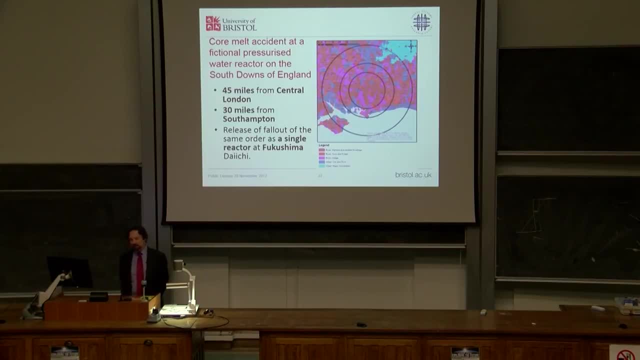 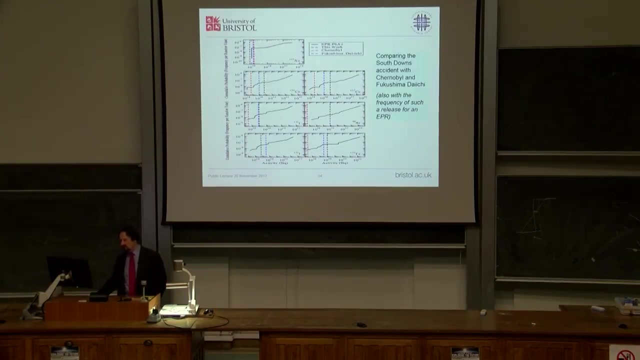 and the release was roughly of the same order as what happened at Fukushima Daiichi, from a single reactor. so it's about a quarter of what was actually what actually emerged from Fukushima Daiichi. and when I say similar, this diagram, which I guess is a bit busy actually, but if we concentrate on the, the vertical, 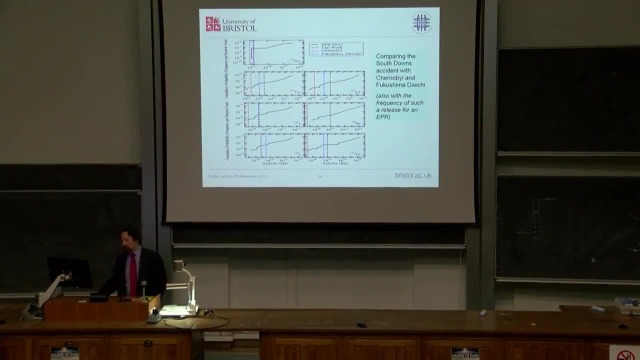 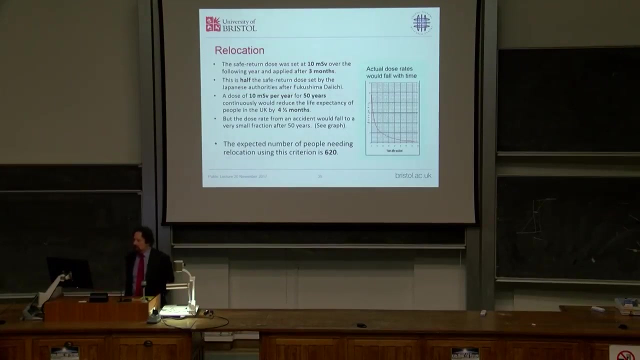 lines there: the black vertical, black dotted vertical line and the blue vertical line is looking at a number of ice, of radioactive isotopes, and if you divide the blue by four, you more or less in most cases you get the what, what was actually looked at very roughly at on the South Downs reactor. for this, the, the. safe return dose was set at 10 millisieverts over the following year and applied three months into the accident. so if the the safe return dose was set at 10 millisieverts over the following year and applied three months into the accident. so if the 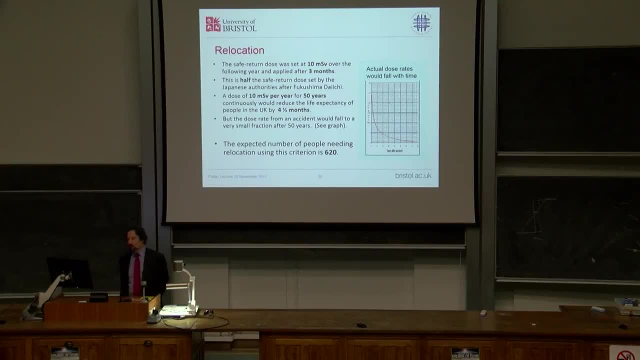 if anyone, if the dose was going to actually go, was not was was higher than 10 millisieverts over the over 12 months was calculated to be, then you don't return. that's actually half a dose that the, the safe return dose that the Japanese authorities used. and again to put that in context, if you actually receive a dose of 10 millisieverts per year for 50 years, that will reduce your life expectancy by four and a half months. so there are a hundred thousand homes in the UK that face that as a matter of course as a result of radon seepage. so it is. it is a pretty low dose, and and 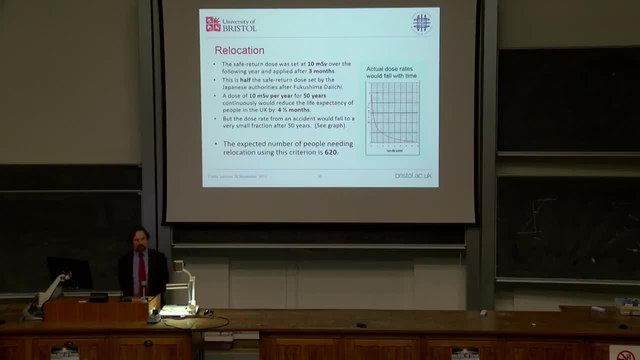 remember that you wouldn't be getting a constant dose. the dose be falling as the red line on the graph indicates there, but when that was put into, it is rather strict return research. so the average number that you would expect from such an accident on the South Downs of England, 45 miles from central London. number of people needing. 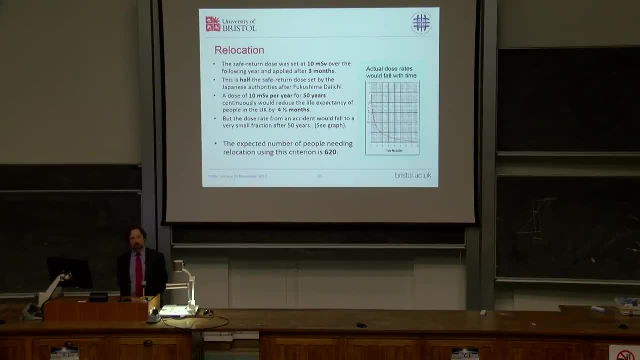 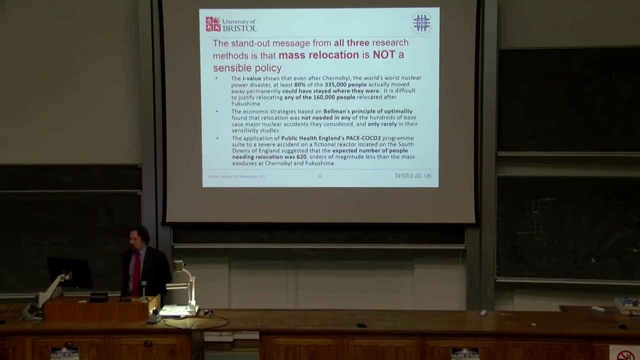 relocation would be 620, I think. you can see this is rather different from three hundred and thirty-five thousand and it's rather different from a hundred and sixty thousand people. so now we're starting to come to think about some conclusions from this and mass relocation. it should not be the policy, the default policy, as it has been in the 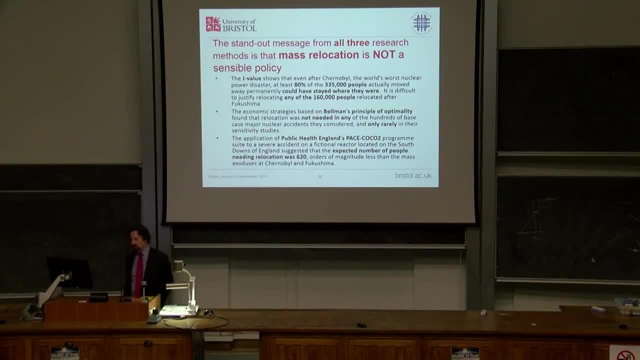 past idea that you should do this. it's in every case, all these things are saying: well, it's not impossible that you will want to relocate your home and you can't. just it's not impossible that you will want to relocate your home, or your home in ever. 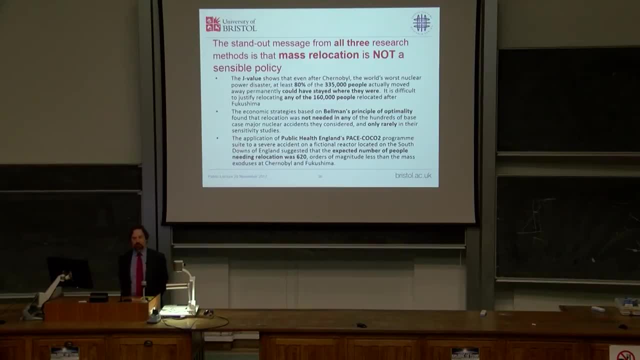 case, all of these things are saying: well, it's not impossible that you will want to relocate some people, but the number is likely to be small and in many cases, don't relocate anyone at all. After a big nuclear accident where the core has melted and there has been a significant release of radioactive- very significant. 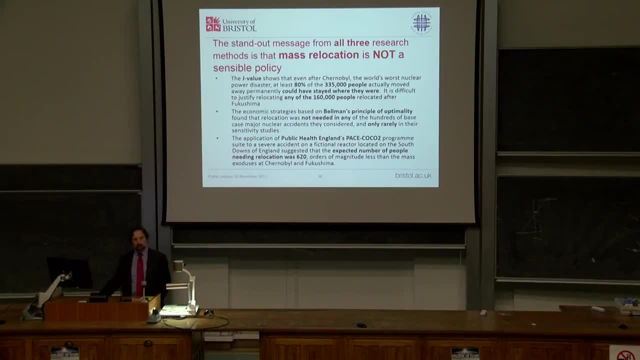 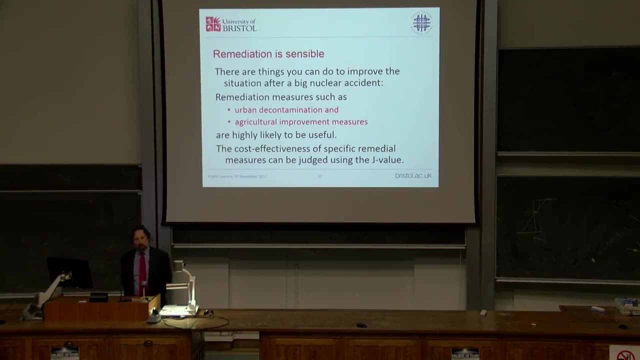 release of radioactive fallout into the atmosphere and the surrounding area. Remediation is sensible and there are certainly things you can do to improve matters after a big nuclear accident and the way to judge those is to use the J value and you can judge whether it is a sensible idea and certainly as far as 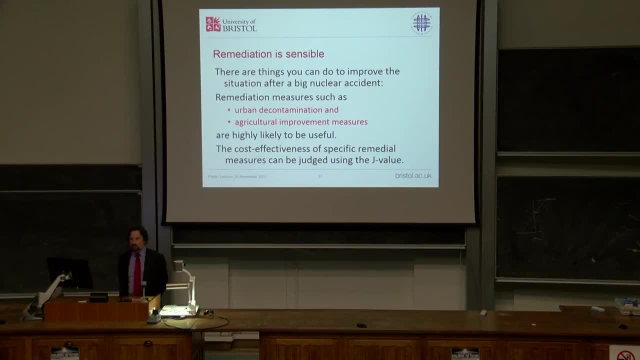 remediation is concerned, some measures which we judged, even 20 years after the Chernobyl accident, were coming out, as I mentioned before, as sensible. Yes, let's go ahead, do it. The total cost of an accident. Well, if the accident is managed in a sensible way. 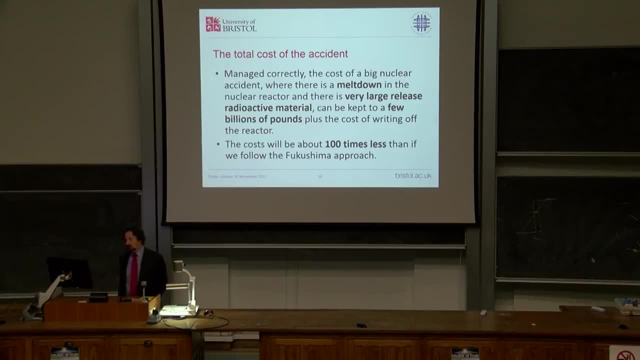 it's likely, the cost of the accident is likely to be a few billion pounds, plus the roughly similar cost of writing the nuclear reactor off as well. That's what the cost should be, so measured in single failure, single figure, billion pounds. but if the example of 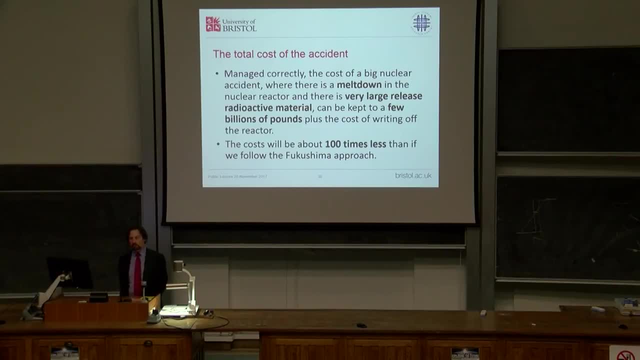 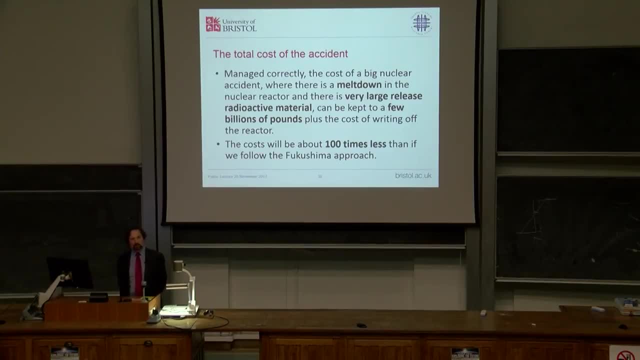 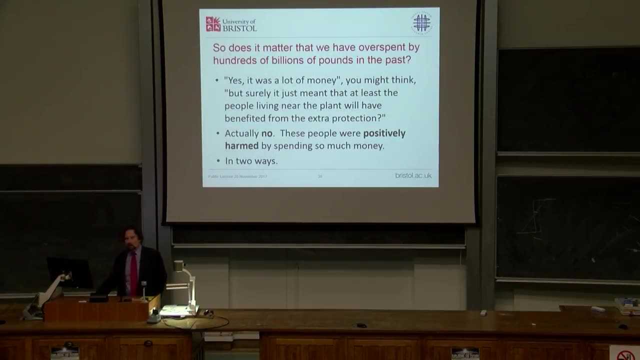 And you're looking at a hundred billion pounds, billion pounds, 200 billion pounds, 400 billion pounds, that sort of order. now i'd like to address the follow-on question from that. so does it matter if we overspend by hundreds of billions of pounds? maybe you think, well, surely it must have helped somebody, it must have helped at least the people. 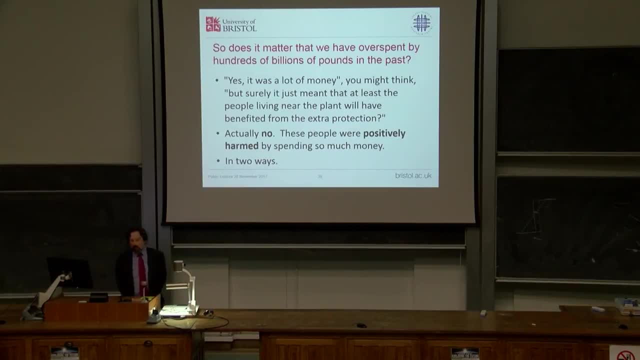 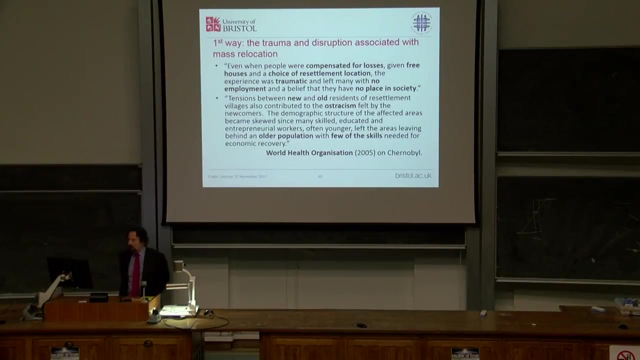 we've overspent, but we're helping the people who are living near the plant because they got this extra protection. no, it doesn't work out like that. there was positive harm done to these very people on whom this money is purported to have been spent. we know that because we have world health organization reports. which tell us that even when people compensated for loses, given free houses and a choice of resettlement location, the experience was traumatic and left many with no employment and a belief that they have no place in society. tensions between new and old residents of resettlement villages also contributed to. the ostracism felt by the newcomers. the demographic structure of the affected areas became skewed, since many skilled, educated and entrepreneurial workers often used to have an younger left the areas, leaving behind an older population with few of the skills needed for economic recovery. that's the first way, but that's not the only way in. 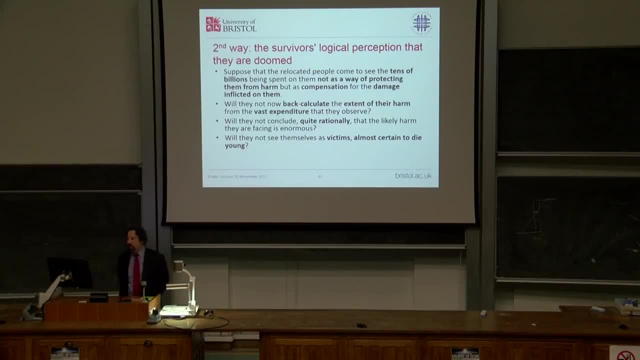 a sense, that's the obvious way. the second way is the survivors perception- and it's a logical perception- that they are doomed. suppose that the relocated people come to see the tens of billions or hundreds of billions of pounds that have been spent on them, not as a way of protecting them from harm, but as 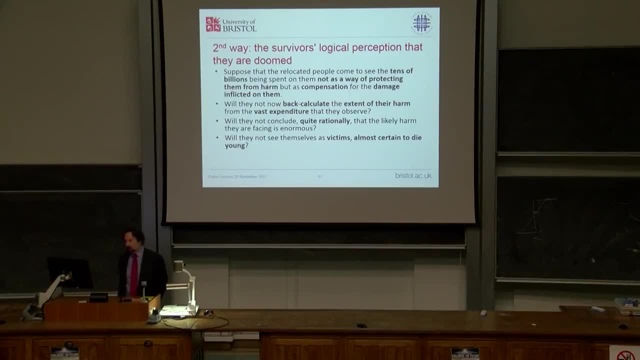 compensation for the damage has been inflicted on them. they see themselves now as victims, won't they now back calculate the extent of their harm from the vast expenditure that they observe? they may not understand the units of radioactivity and radioactive dose, but they certainly will understand when huge 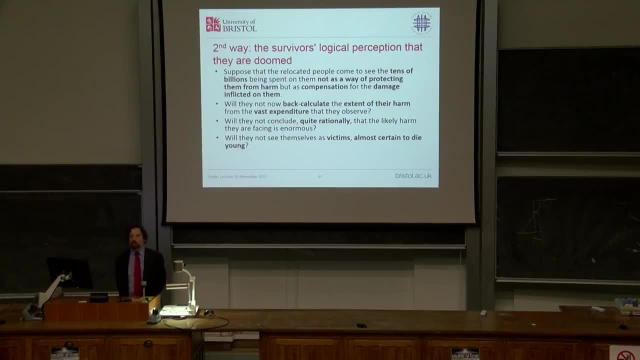 vast sums of money are being spent. so why is the government? the government's never spent that amount of money on me before. why is it doing that? doing it now? I must be in a truly bad way. that's the logic, you know, and they see themselves as victims almost certain to die young. 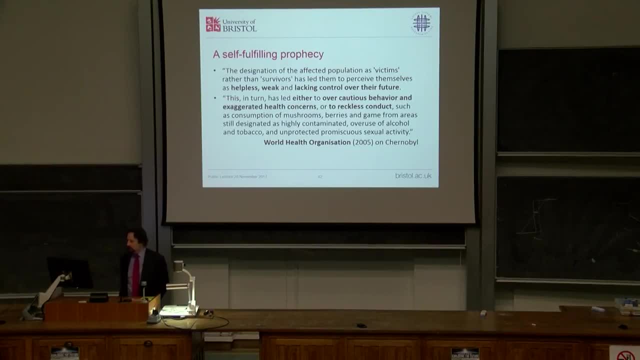 again the World Health Organization. the designation of the affected population as victims rather than survivors has led them to perceive themselves as helpless, weak and lacking control over their future. this, in turn, has led either to overcautious behavior and exaggerated health concerns, or to reckless conduct such as consumption. 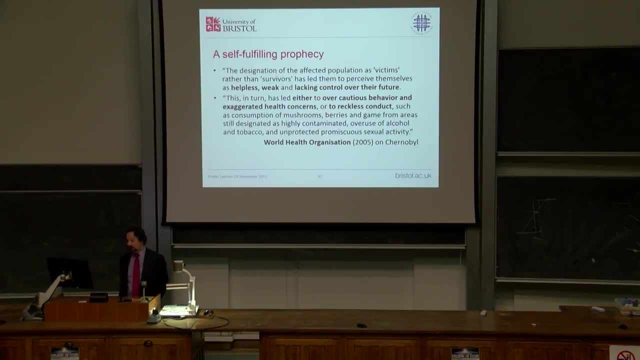 of mushrooms, berries and gain from areas still designated as highly contaminated, overuse of alcohol and tobacco and unprotected promiscuous sexual activity. I think a comment that that needs to be made there is they that they now perceive themselves as destined to die young. that's not a nice state for anyone to be in. 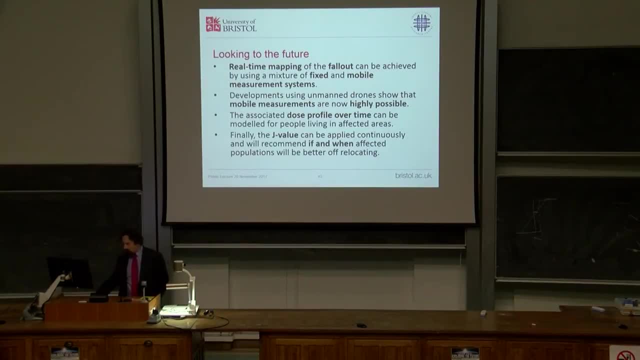 so I think we've gone down the road of reading metaphors and we will leave there child and mother. this is, these are the two questions at this very important point. I think the first conclusion from from this which has come out from this is that relocation should not be the obvious policy of 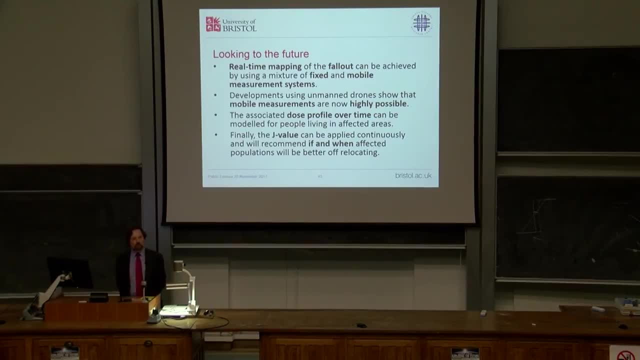 choice. we know that now and even if we had no further information, we would be said we should be very hesitant about employing mass relocation after a bigis. in both cases, the relocation option was not. the was exaggerated in the. in the case of Fukushima, exaggerated completely, but we would like more information to 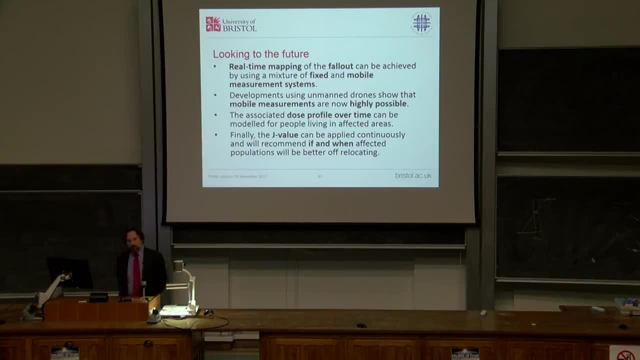 guide the decision-makers early on, and this is indeed possible. so, looking to the future, if we look towards real-time mapping of the fallout using a mixture of fixed and mobile measurement systems- and here work at Bristol has shown that unmanned drones are now highly possible in order to give mobile measurements- we 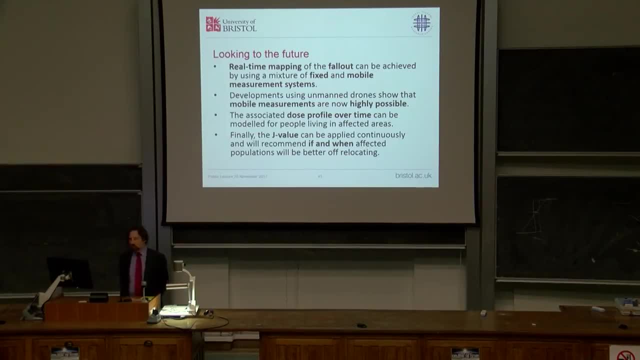 can feed that into a model and we could no doubt improve the models that give the dose profile over time. not only from the ground shine, from the radiation, but also from the food ingestion. and we can, we can develop those and use those and then we can apply the J value. 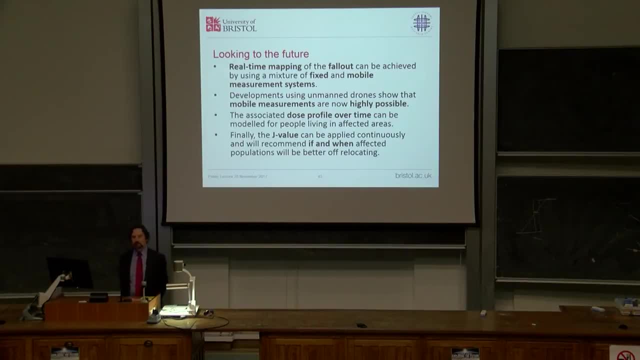 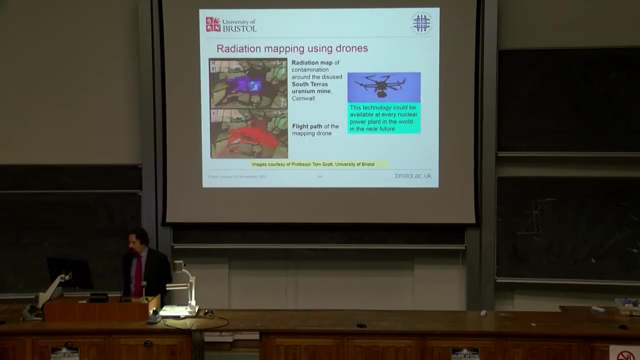 continuously as the accident develops, given we've got one of these very unpleasant big nuclear accidents actually happening. but we can now supply the decision-maker with information so that the Japanese Prime Minister does not have to consider evacuating Tokyo. World's first saltwater missions hotel is located around the Bay of Scots and 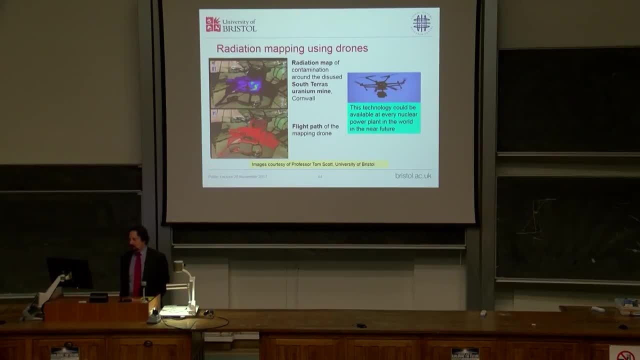 it's 249 miles from the capital. the saltwater mission is only 25 miles from the national airport and we've just analysed the different examples in the survey and we have a third-party report of the many incidents over in vielleicht, as some might be from another. 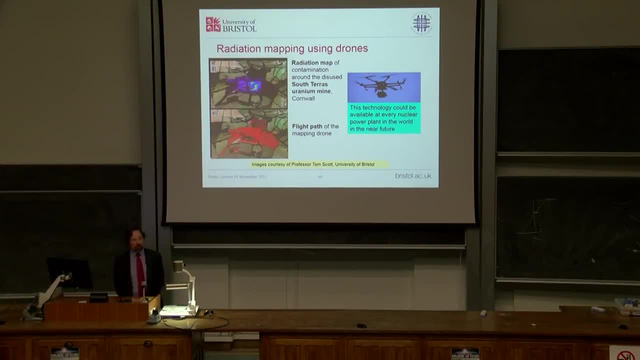 region in Scotland, and one of them in this region is aุ. well, that is an incredible photograph at the moment and it's this media wrap-up against the graveyard of some of the most. instead, this place in the paste topline has been pleasantly weakenulture from world to a rich childcare artist下來 itобu s.